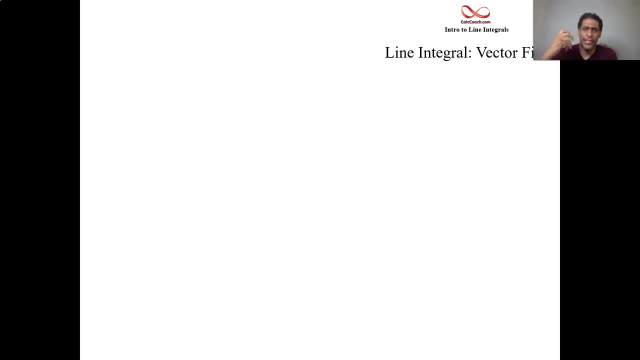 Hello, welcome in this video. What we're going to do is look at the line integral from the vector field perspective. Remember, the vector field is a slope field. It used to be called back in your previous calc class, where you have a bunch of arrows that represent a vector function. 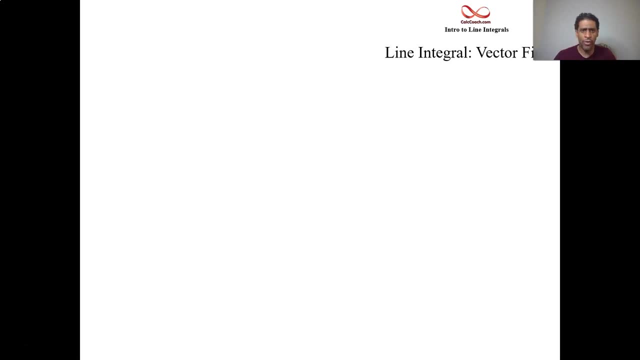 You give me an X and Y, I give you an arrow. The arrow is then going to be represented by a direction And then, as far as magnitude, it's going to be hard to actually represent that, because some have a larger magnitude than the others. 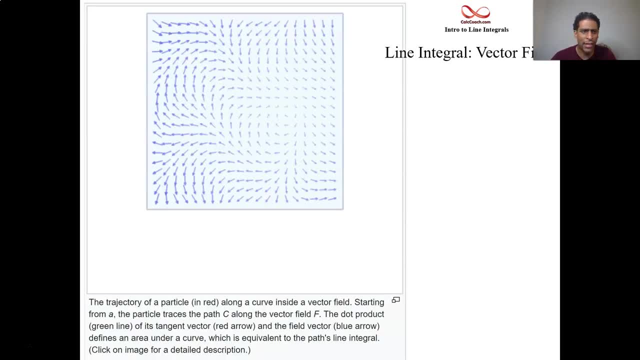 And so we're just going to maybe represent that with bolder arrows. And so here's an example of a vector field. This is once again straight from Wikipedia And the visual. now, as to what are you measuring When you change perspectives, when you start looking at a vector field- line integral as opposed to a scalar function- line integral- what are you measuring? 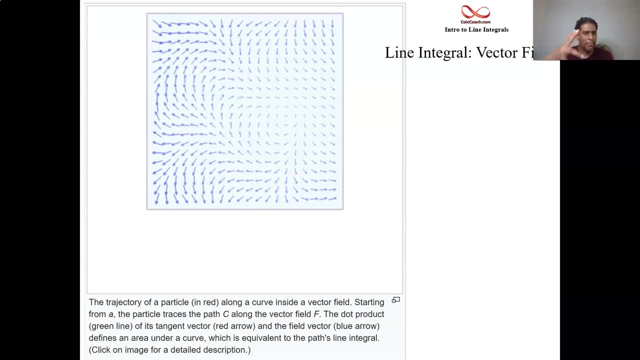 Well, in this video you'll see an animation that will take place And the idea is that there is a particle who is on the curve at a starting point and an ending point And you are calculating the work done by the vector field to move the particle along the path. 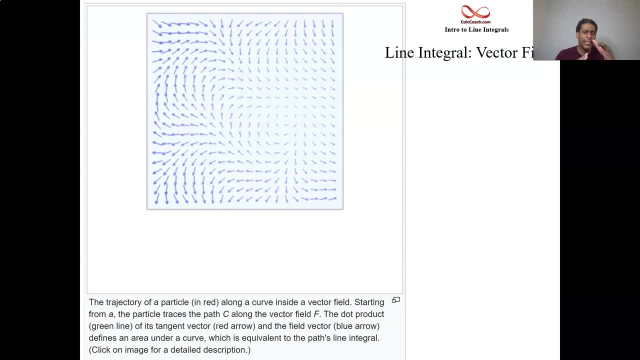 You're doing a dot product with the vector field and the tangent vector to the curve. The video should play now. So we have our vector field And we have our curve. If I could pause the video, that would be great. I can't pause the video, That's okay. 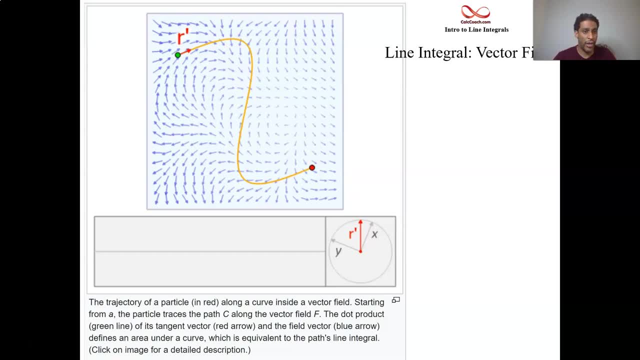 And so We have: the red vector represents the tangent vector, and it's an accumulated dot product. as we traverse throughout the curve, When the vector field is pointing in the direction, then they're going to be parallel to each other, And so the dot product between the vector f and r prime is then going to be equal to. 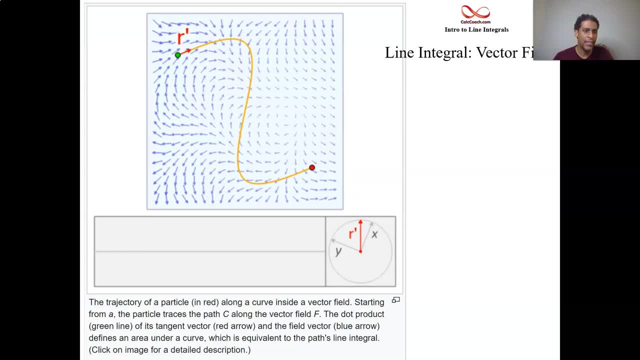 Just the magnitude of the vector field. It's when Let's see if I can stop it at the right point. No, I can't start and stop it. All right, so just watch it. I might have to go back and play it again for you so you can see it. 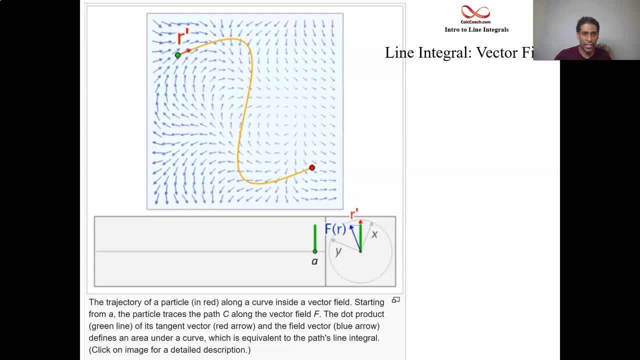 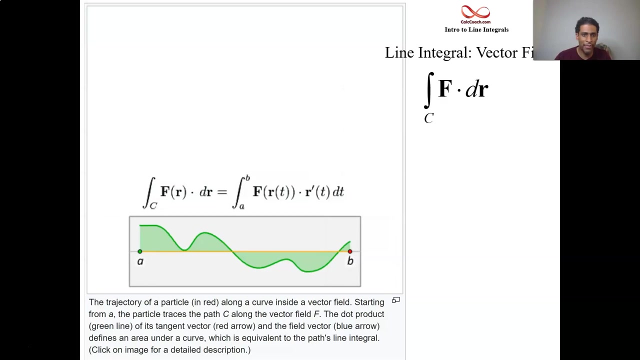 But watch as you go down. Watch the dot product value be equal to zero As the vectors are orthogonal to the curve. Can I go back and play that again? Let's explain. We'll explain that later. but No, Okay, it'll play again. Here we go. 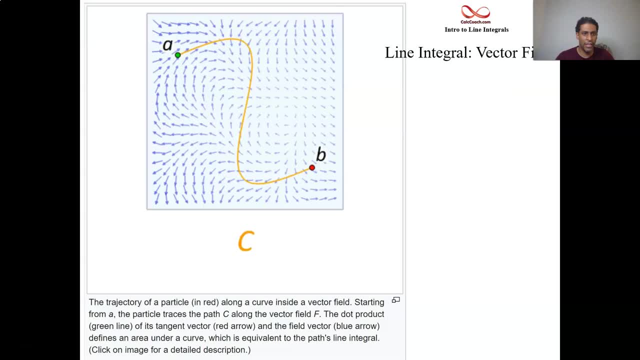 So we have the vector field, We have a curve, We have the red vector. who's going to represent the derivative curve down in the circle there? The blue vector is going to represent the vector field. The red vector is going to represent the vector field. 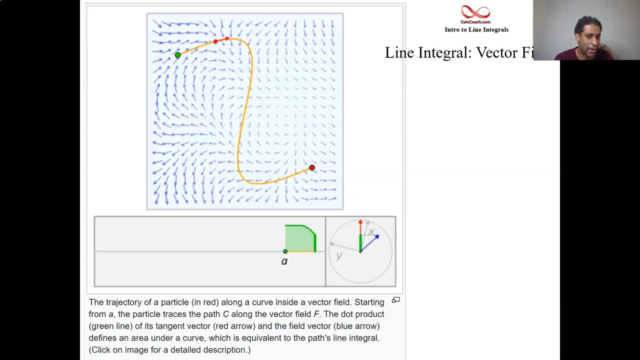 And we are doing dot products And the green value is the dot product. Zero, Zero under It's negative. It could be negative, right Dot product could be negative And it's all about the angle that you're making with the tangent vector. 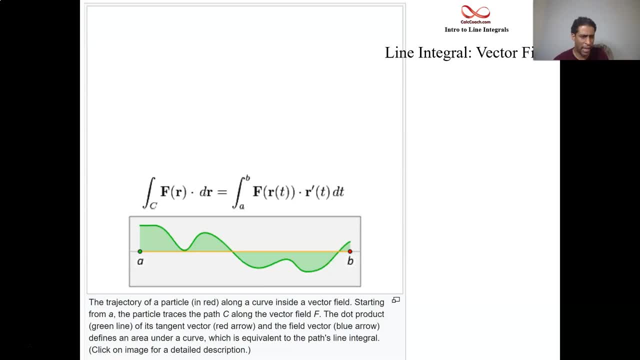 Cosine of the angle is going to be what comes from dot product. And so when the cosine is something that is less, When the angle is something between zero and pi over 2. Cosine is positive. But when the angle is something between zero and pi over 2, cosine is positive. 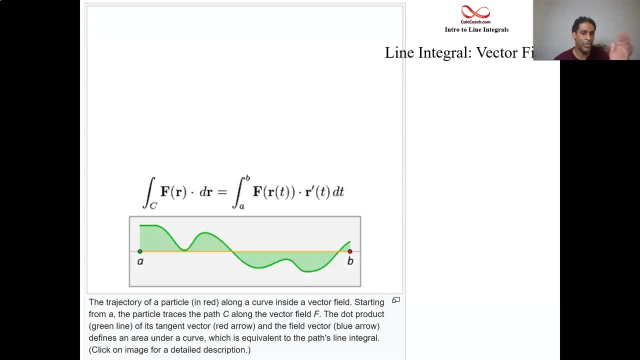 But when the angle is something between zero and pi over 2, cosine is positive, something more than that between pi over 2 and pi, then the cosine is negative and so that's why you saw this guy dip below the graph here, and so negative dot product is possibility we're talking. 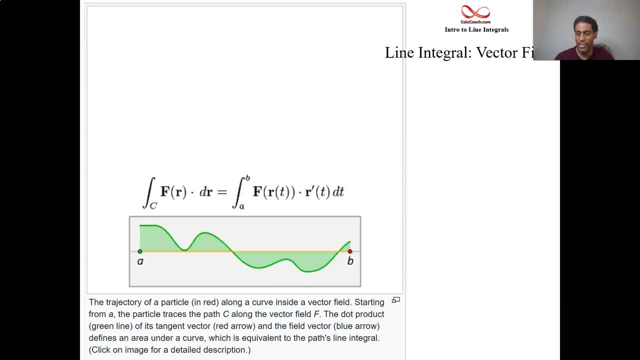 about the net dot product from t equals a to t equals b. the integrals are written with the same integral sign in a, C, but inside that we have f, dr. dr is the derivative of your path, function r, and we're gonna write it in this format, with the f, is a vector who has multivariable functions. 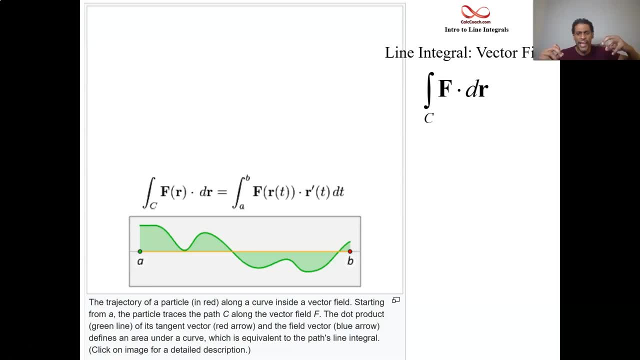 and it as its I and J, perhaps K components and those multivariable functions. we're gonna call them P and Q. all right, and so the P and Q come from F, and then the integer and the derivative of the comma. together, the comma together grows, and so that obrigates Katy Meter's welcome of and. we end up with one block, of vector a, integral sine, grab d, vector dot c, which matches the lambda p integral sine. very well, feet. and the integral sine equals the integral point from k, equal connect. all right, there, we're done. so one more time, let's go back, and then we're also next, we're. 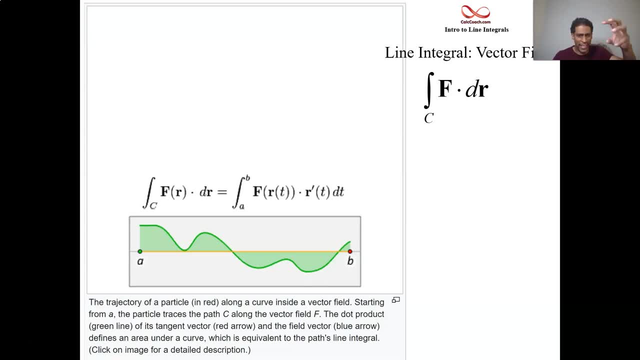 let's go to. what we're actually going to learn is in this our leucheve two: vous for almost. And then, as far as dr goes, r is a vector that has x and y's. x is the i component and y is the j component. functions of t. 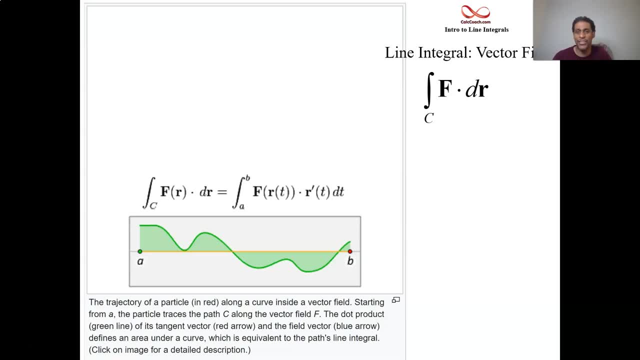 And when we take its derivative we get dx and dy. So if we're dotting, we're going to have pdx and qdy. Our line angles look different than we had before. Before we had a multivariable function, for sure. 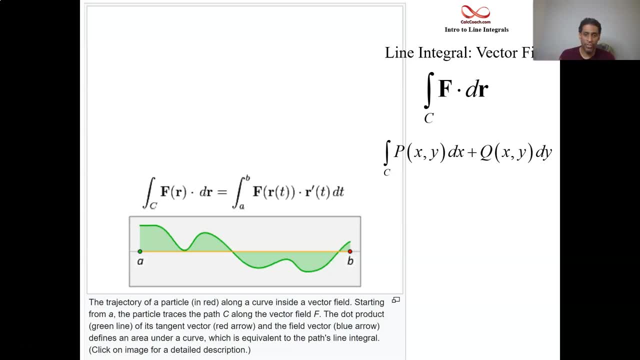 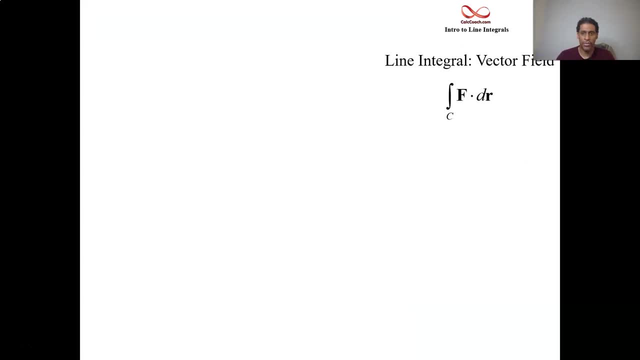 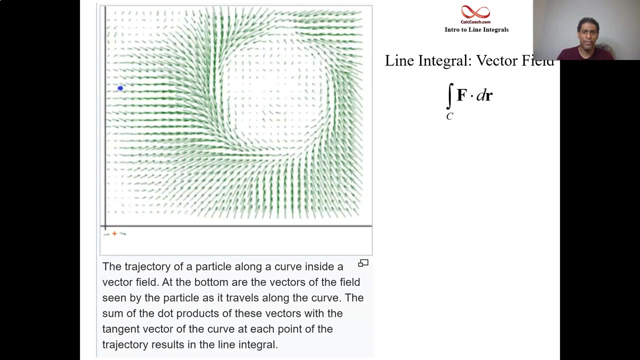 but it was times ds. This is two multivariable functions, one times dx and one times dy. All right, great. Here's another visual, straight from Wikipedia again, where we have a vector field drawn in. The curve won't be drawn in, but at the bottom. 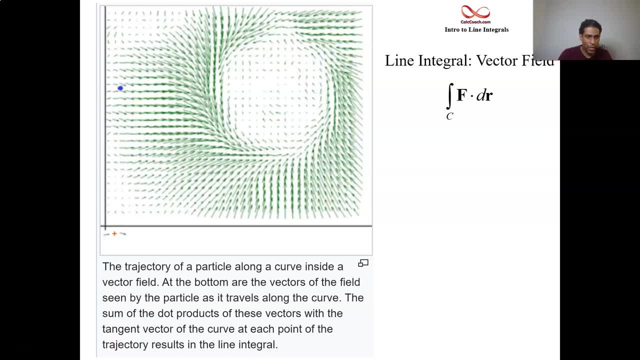 what's nice about this video is that you can see the actual vector that is closest in proximity to the smallest along the curve, close to the blue dot. there the blue dot, The blue dot is the particle and it's going to move along. 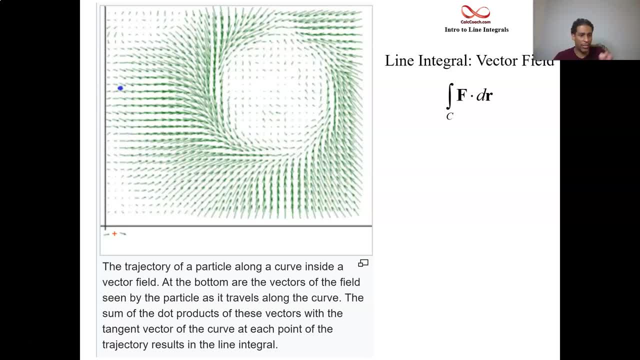 And at the bottom there they're going to draw in that vector as you go and it's going to be plus the other. It's a dot product. You're not adding vectors, no, But you're saying I'm dotting the direction vector. 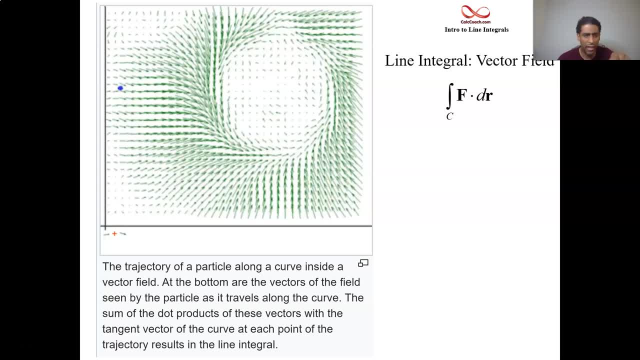 for the function, the derivative of that with the vector field, And so I think the video is going to play now, So the curve isn't explicitly marked off. Oh, there it is, At the end it's finally marked off. 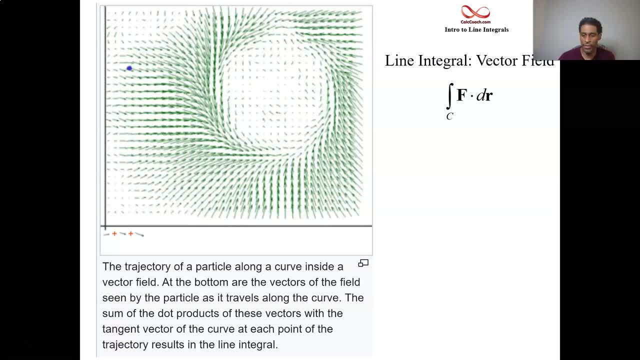 And so it's going to replay. Oh, that's great. Oh, it's not going to replay. OK, let's make it replay by going back. OK, there we go. All right, larger arrows represent a stronger magnitude, And so we're accumulating these vectors dotted. 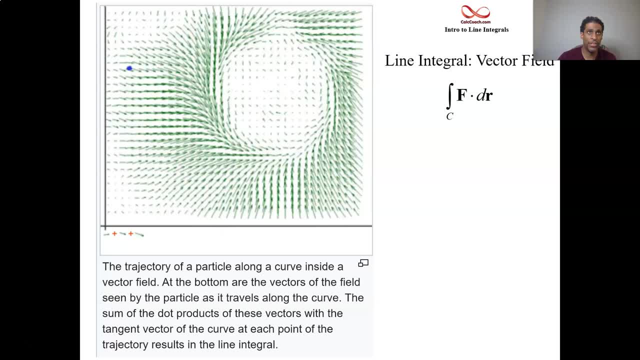 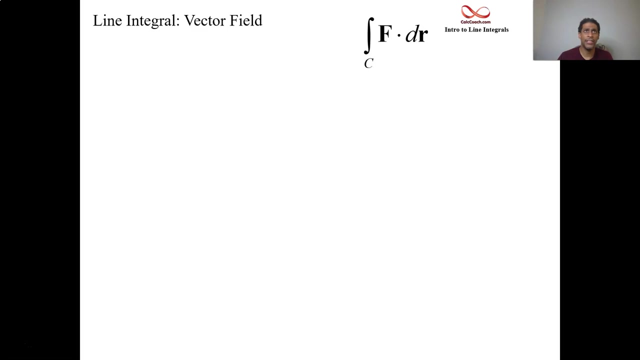 with our velocity vector One more time. All right, great, So we're looking at the dot product, these vectors, with the tangent vector to the curve, at those distinct points there marked off on the curve. All right, great, So that's the visual. 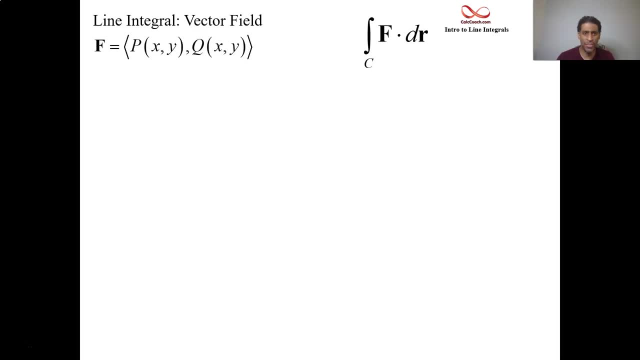 Let's go ahead and tell you the steps And then in the next couple of slides we'll look at some examples. So let's stay with 2D for now. So you have your two elements right: your vector field and your curve. 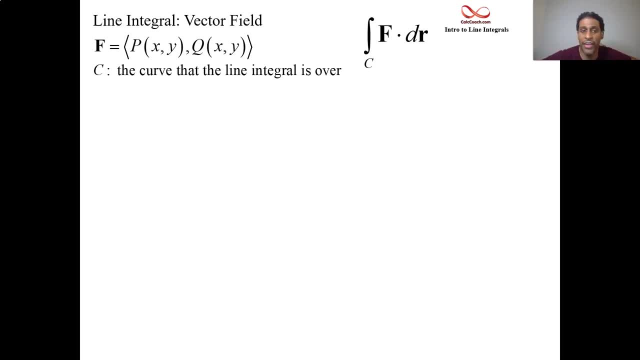 The vector field has these components: p and q, multivariable functions of x and y, And c is your curve, And we're going to execute the line integral over the curve of the dot product between f and dr. Let me give you the steps. 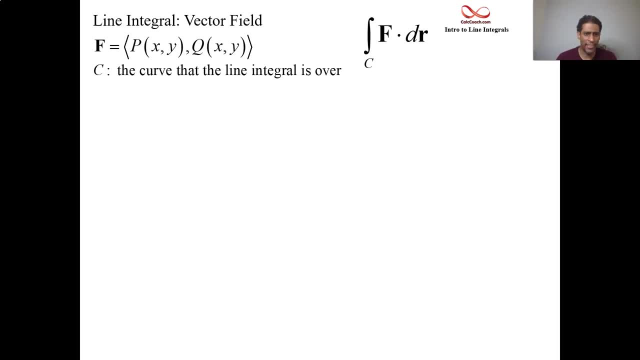 The first thing is to start with the path. let's say, Parameterize the path. All right, we had a video on parameterizing basic paths, So please go back and watch that if you need to. But you need to come up with the functions g of t and h of t. 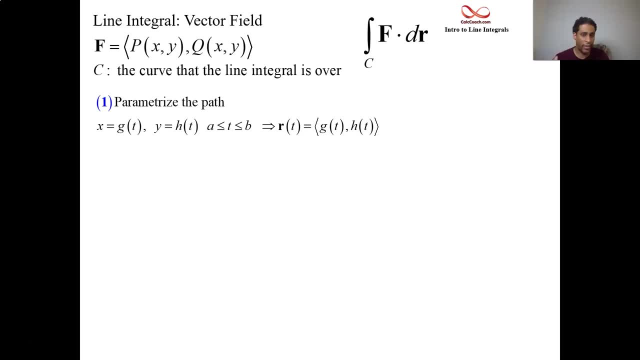 and the boundaries on t that will traverse You exactly along that curve. After you get that path, write it as a vector. Put those guys as components in the vector r of t and find the derivative of the path dr. So just take derivatives g prime and h prime in a vector. 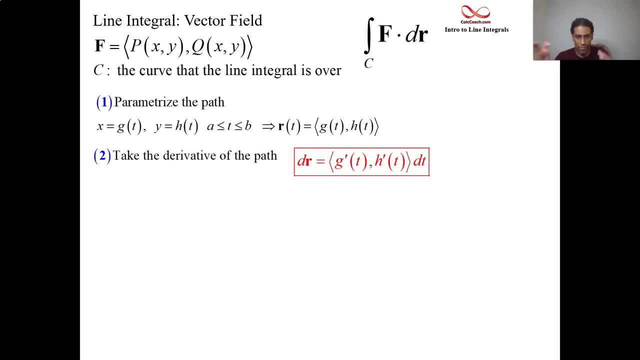 Officially it's g prime of t? dt and it's h prime of t? dt, but we can factor that dt part out. Now that's half the battle right. f dot dr. So what about f? f is going to be this function full of multivariable? 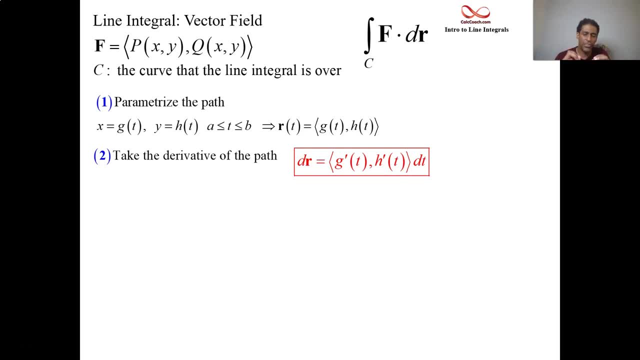 a vector function full of multivariable functions, scalar functions, And when we have our parameterization, we can now rip out all the x's and put in g of t, Rip out all the y's and put in h of t. We're rewriting f. 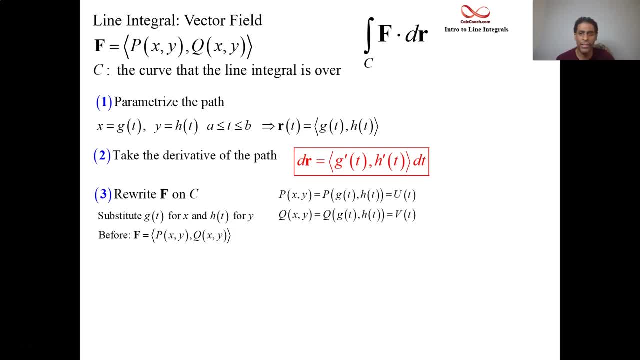 We're restricting f to be only on the curve again. What that's going to then give you is a function in t. A single variable. p is going to be a function just of t. I call it u of t here. q is going to turn into a function just of t. 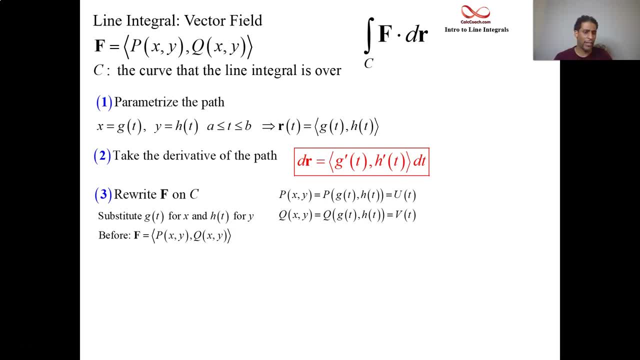 I call it v of t here And what I call it is f on c. It's f rewritten to only be considering the points that are on the curve, And we take a dot in step four, The dot between step two and three.